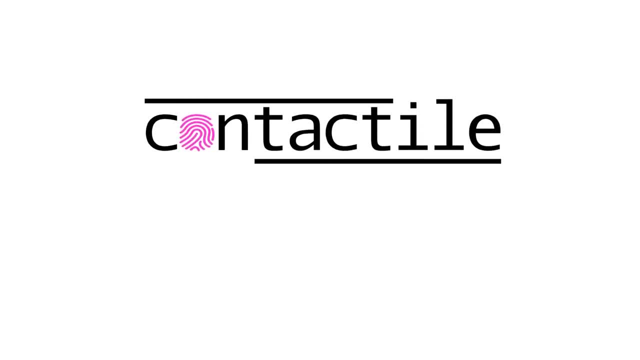 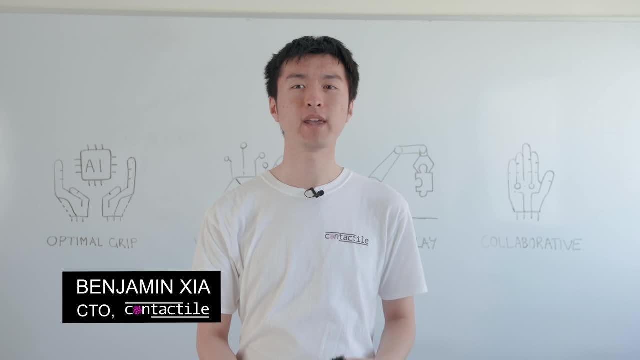 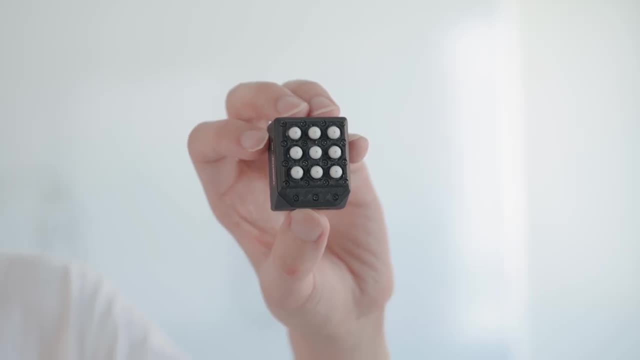 Hi, I'm Ben, co-founder and CTO of Contactile. We're giving robots a human sense of touch and enabling robotic dexterity. Our core product is a revolutionary tactile sensor that measures all the same tactile parameters as the human finger. Here we've got two of our tactile sensors mounted. 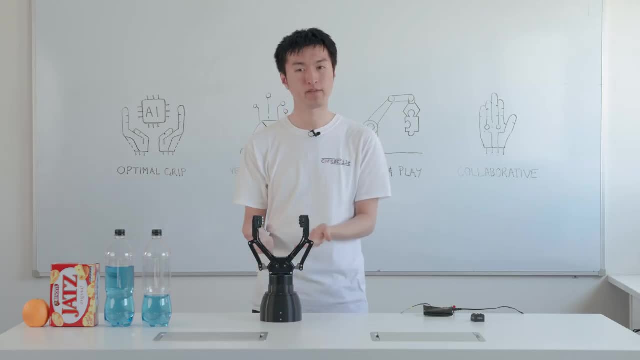 to this standard off-the-shelf robotic gripper Without the feedback from our sensors. even the best robotic grippers in the world today still have to be pre-programmed for any object they're expected to pick up. So, for example, if I wanted a robotic gripper to pick up this bottle, I'd have 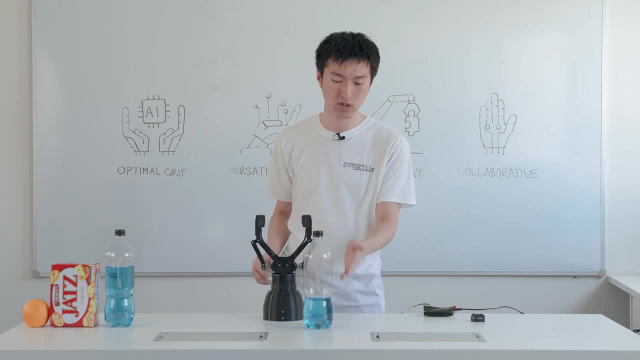 to know in advance exactly how hard it needs to squeeze to stop the bottle from slipping out of its grasp. So in this case I've pre-programmed our gripper for this particular bottle. So if I attempt to pick it up, you can see that I'm able to lift the bottle. However, if there's any sort 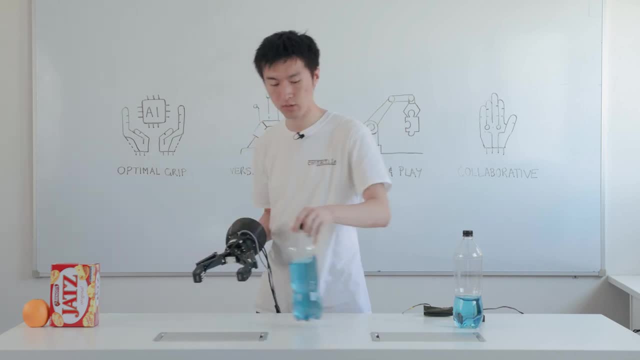 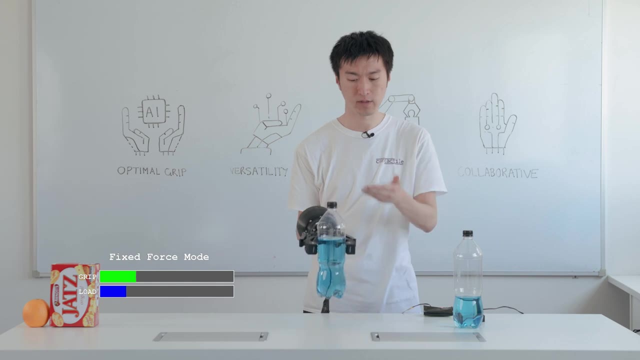 of variation or unknown parameters in the robotic gripper, I'm able to lift the bottle. But if I want to pick up a bottle that's not as heavy as the object we're trying to handle- say, for example, if it were to be heavier than expected- then suddenly those same pre-programmed 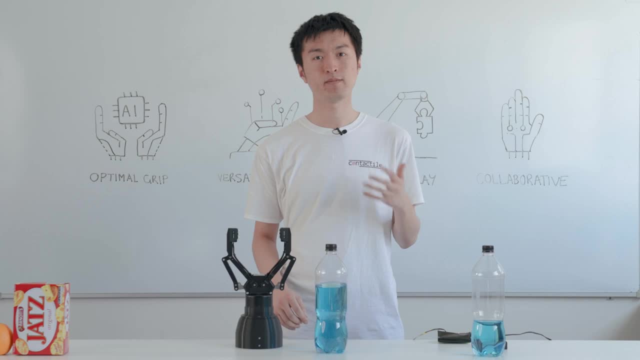 parameters may no longer be sufficient. As you can see, the bottle is slipping straight out of my grasp Now. this kind of manual handling task is very simple for a human to do. If you got any person and blindfolded them, told them to pick up this bottle the moment they touch the object and 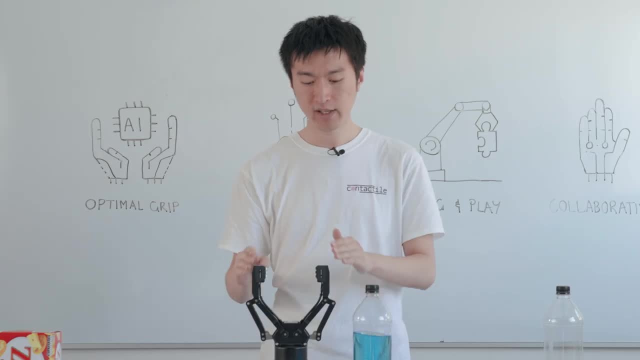 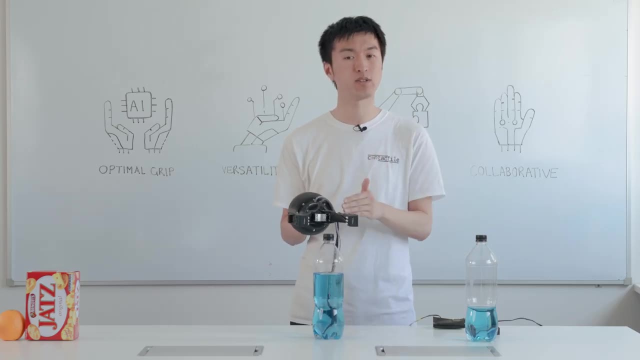 attempted to lift, they'd be able to feel exactly how hard they need to squeeze to stop it from slipping. With the feedback from our senses, we can give this robotic gripper the same human sense of touch. In this case, with the feedback from our senses enabled, all I need to do is tell the gripper to. 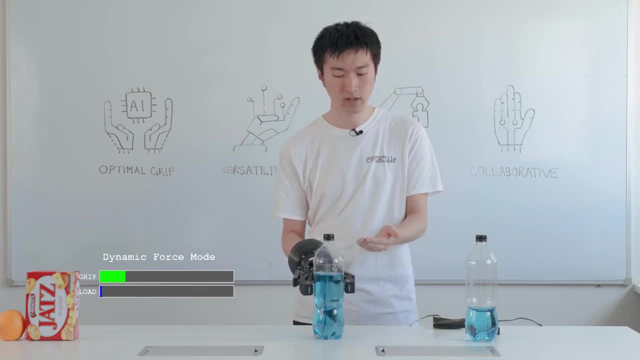 grip and upon making contact, it can feel exactly how hard it needs to squeeze to prevent the bottle from slipping. And this is working in real time. So even if there are dynamic loads- for example, if I were to increase the weight, it would increase the force If I decrease the weight. 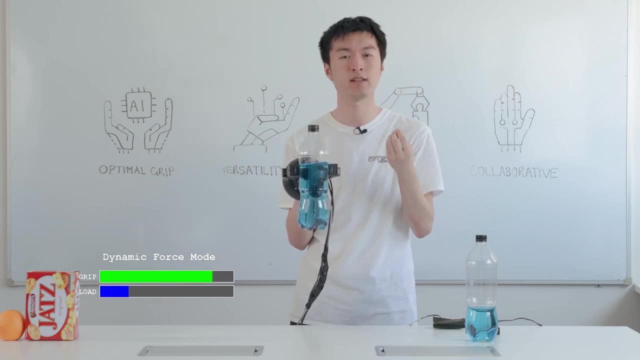 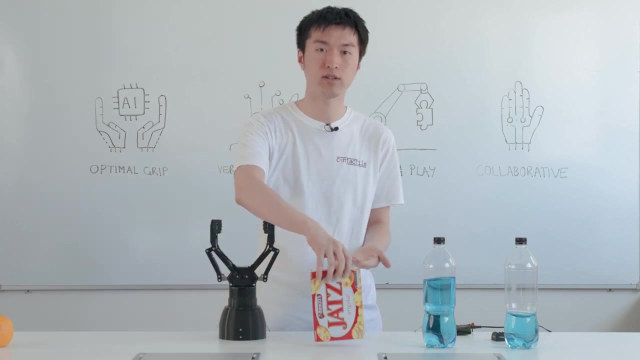 it will decrease the force because it knows exactly how hard it needs to squeeze. This is very useful in any situation where we might have an object that's crushable by excessive grip forces. So, for example, if I want to pick up this box of biscuits, all I need to do to tell the